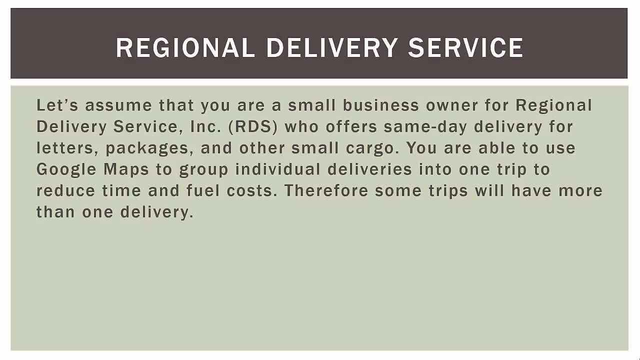 So let's assume that you are a small business owner for Regional Delivery Service Incorporated, or RDS for short, who offers same-day delivery for letters, packages and other small, small cargo. You are able to use Google Maps to group individual deliveries into one trip. 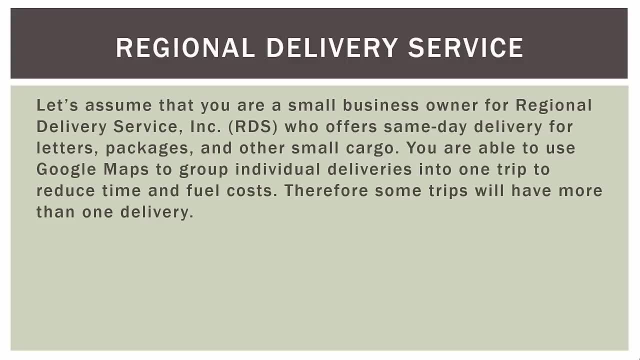 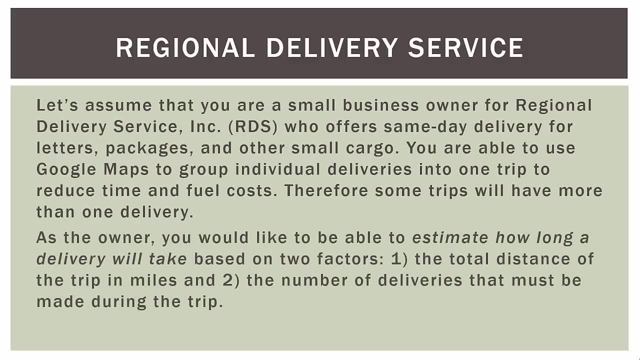 to reduce time and fuel costs, just like UPS would, or FedEx or the Postal Service does. Therefore, some trips will have more than one delivery. Now, as the owner, you would like to be able to estimate how long a delivery will take, based on two factors. 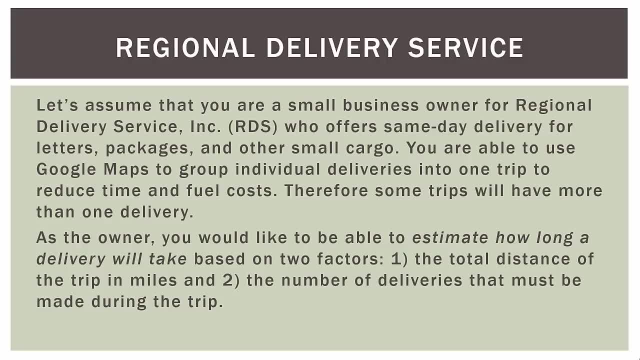 One, the total distance of the trip in miles and two, the number of deliveries that must be made during that trip. So we're looking to estimate how long a delivery trip will take, based on the distance and the number of deliveries during that trip. 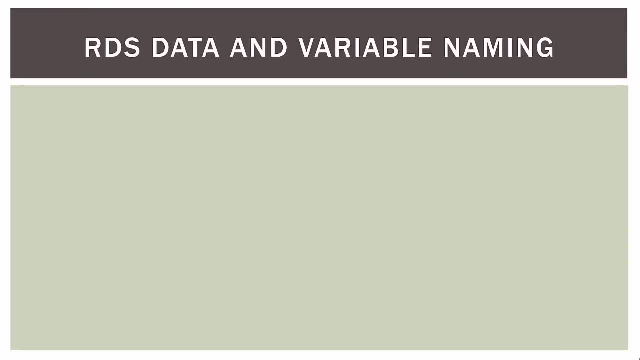 So two factors. So to conduct your analysis, you take a random sample of 10 past trips and record three pieces of information for each trip. One, the total miles traveled of miles traveled. two, the number of deliveries during that trip. and three, the total travel time. 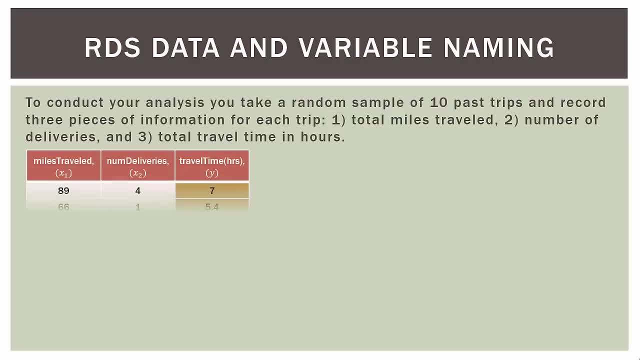 in hours, which is what we're trying to predict. So you make a table that looks like this: So we have miles traveled, num deliveries, which is the number of deliveries, and then travel time in hours. along the top We have labeled them x1,, x2, and y. 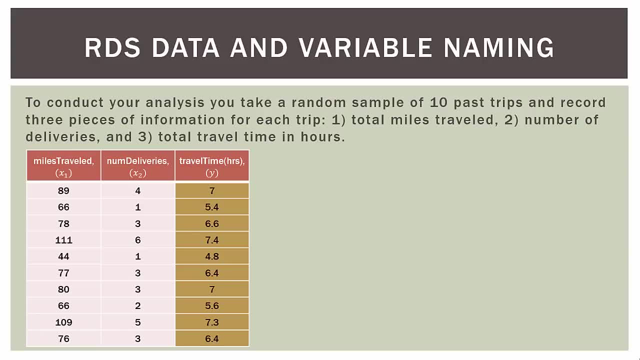 Now, x1 and x2 are special types of variables we'll discuss here in a minute, and y is a distinct variable we'll talk about here in a minute. So we can see the first trip. we traveled 89 miles. we had four deliveries on that trip. 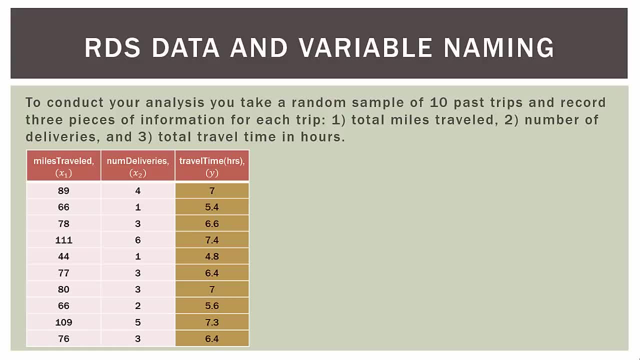 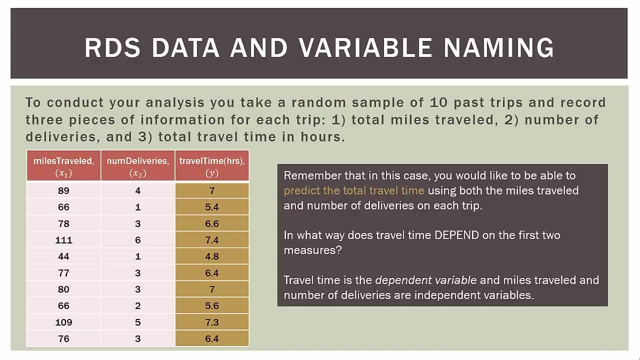 and the total time was seven hours. The second trip was 66 miles, we only had one delivery and the travel time was 5.4 hours. So here are our 10 trips. Now remember that in this case, you would like to be able to predict. 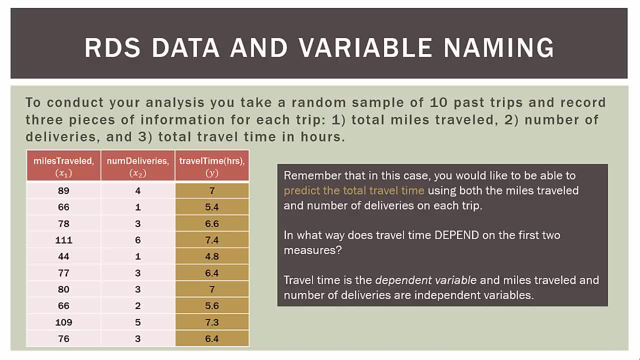 the total travel time. So that's the right column, sort of in the orange-brown color there, Using both the miles traveled, which is x1, the first column, and the number of deliveries, which is the second column- x2, of each trip. 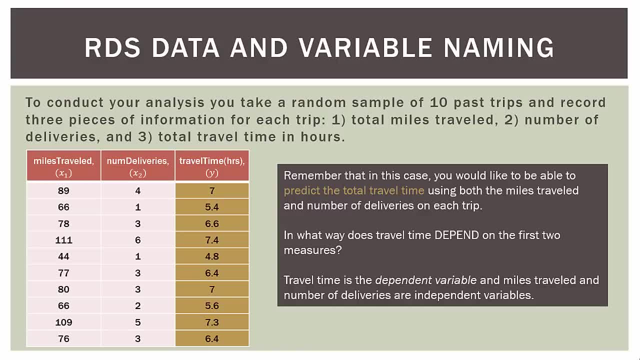 So the question is: in what way does travel time depend on the first two measures: miles traveled and number of deliveries? So travel time is the dependent variable, And miles traveled and number of deliveries are independent variables. Now one note here: some prefer predictor variables. 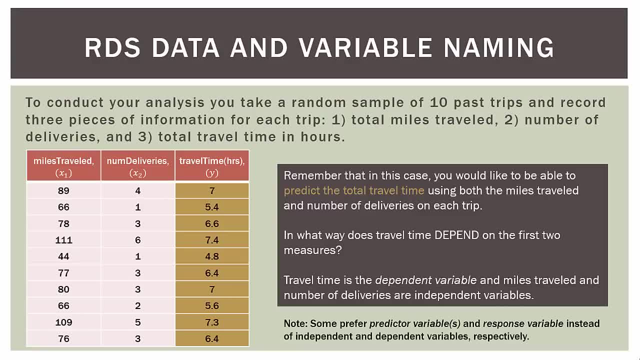 and response variable instead of independent and dependent variables respectively. Since most stats textbooks use independent variable and dependent variable, I am going to stick to that. But I do subscribe to the case of predictor variables and response variable. Just keep in mind that, depending on the text, 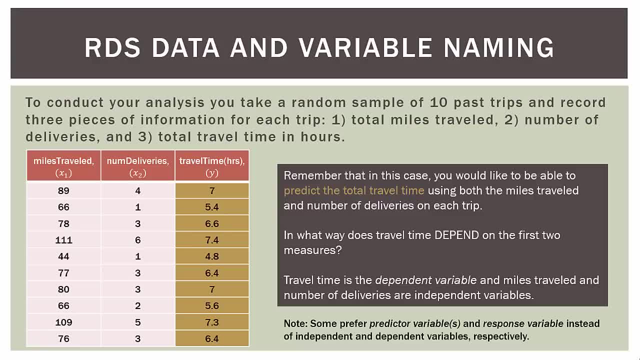 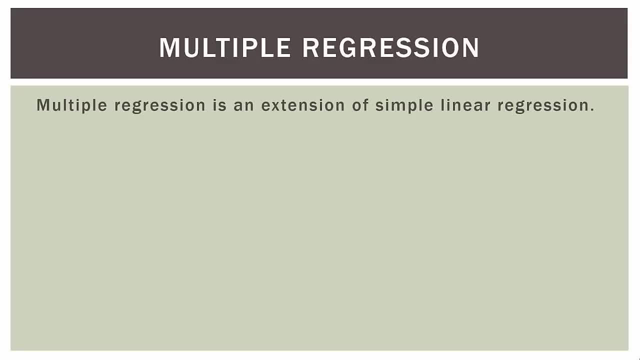 the textbook you're using and your professor and things you may hear, both or one or the other. So what about multiple regression? So multiple regression is just an extension of simple linear regression, again which we talked about in the last series. So remember, in simple linear regression. 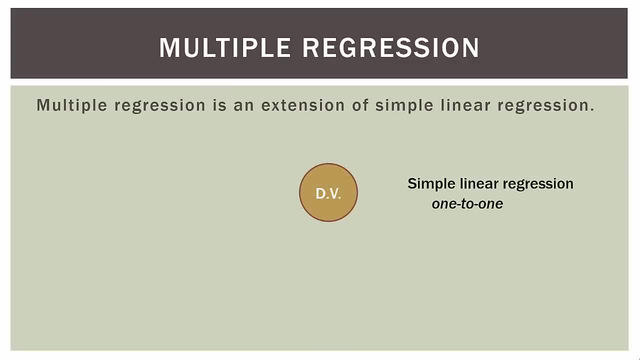 we have a one-to-one relationship. So we have a dependent variable and we're going to utilize an independent variable to explain the variation in that dependent variable or make predictions about that dependent variable. Now, in multiple regression, we have a many-to-one relationship. 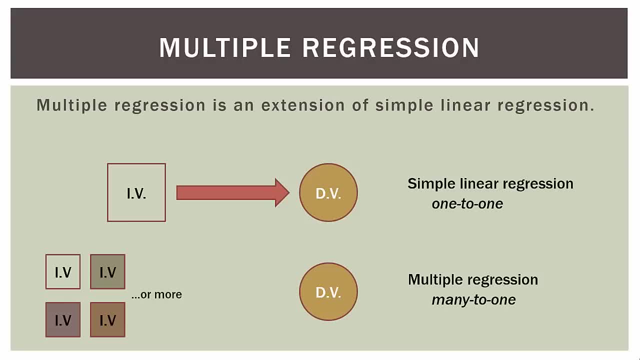 So we still have one dependent variable, but we can have two or more. So in this case we have four on the screen, but we could have more than that, or just two or three or whatever independent variables that are all being utilized to explain the variation. 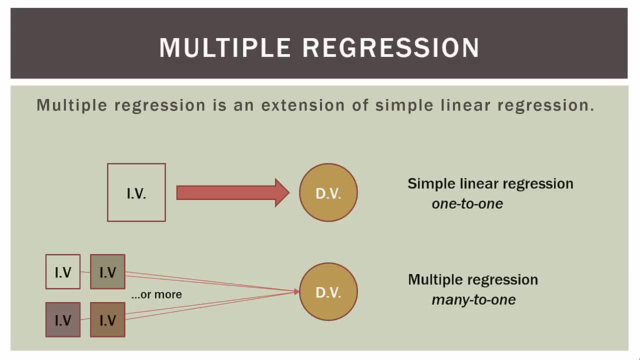 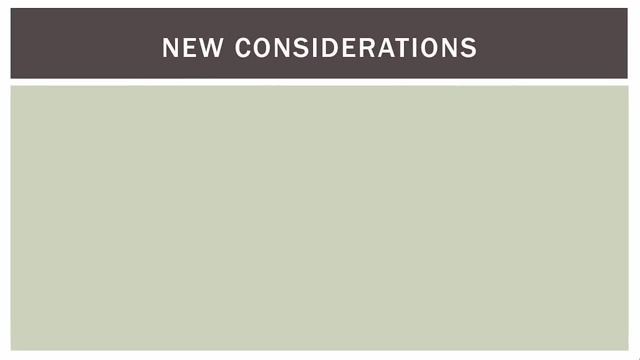 or predict the value of the dependent variable. So we go from a one-to-one relationship, one independent, to one dependent, to two or more independent variables and one dependent variable. Now, having more independent variables complicates things a bit, So we have to have some new things to consider. 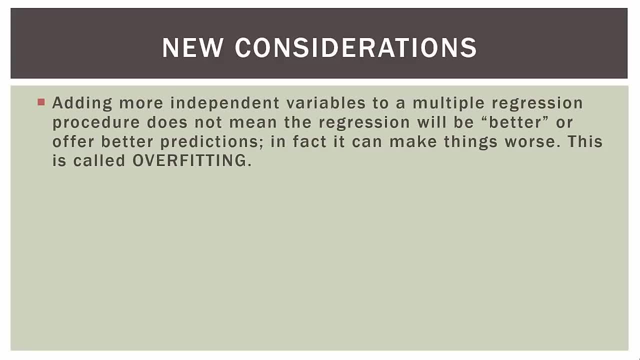 The first is that adding more independent variables to a multiple regression procedure does not mean, or necessarily mean that regression will be better or offer better predictions. In fact, doing so can actually make things worse. This is called overfitting. So let's say we conduct a multiple regression procedure. 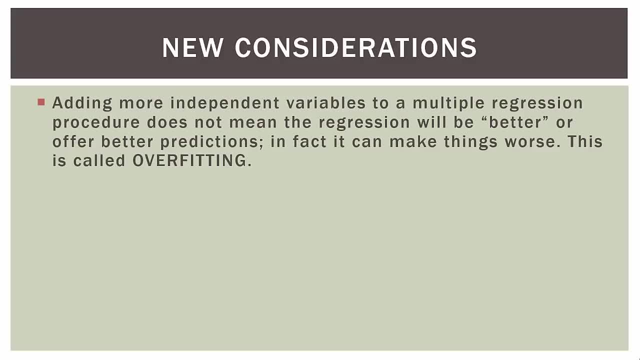 and our model explains 65% of the variation in the dependent variable. Well, for some reason, we don't like that. We think, well, we can do better than that, So we start adding in more independent variables. Well, adding more independent variables will explain. 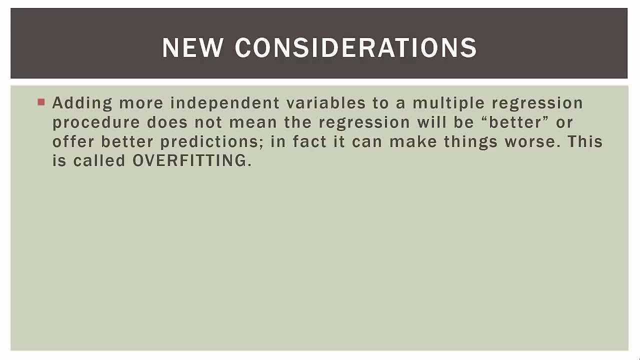 more of the variation in the dependent variable, but it can do so under false pretenses. So adding more variables will always explain more variation, but it can open up a whole Pandora's box of other problems that we definitely want to avoid. So we'll talk about that more as we go. 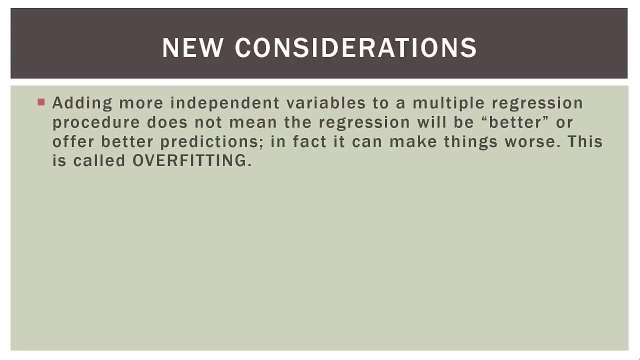 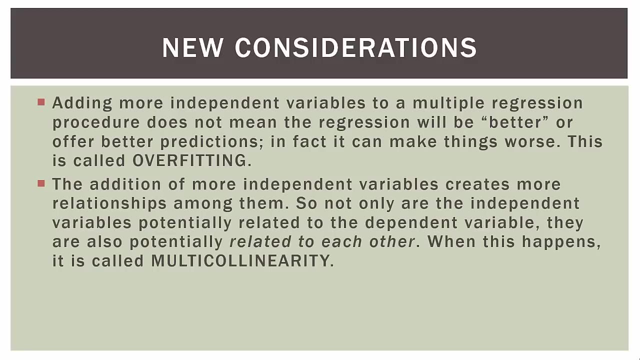 but I just want to float it out there that dumping more variables into a multiple regression procedure is not the way to go. The idea is to pick the best variables for the model. We'll talk about how to do that in future videos. The other concept is that the addition 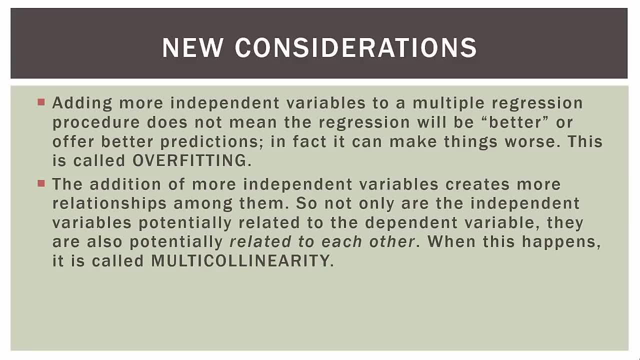 of more independent variables- see a pattern here- creates more relationships among them. So not only are the independent variables potentially related to the dependent variable, they are also potentially related to each other. Now, when this happens, it is called multicollinearity. 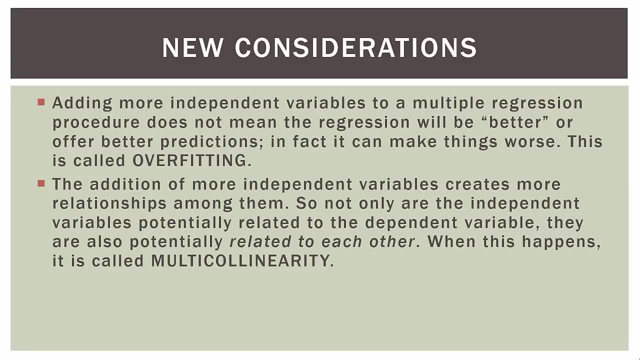 Now, that's a broad term. It's a broad term, A mouthful of a word to say, and I stumble over it sometimes, but hopefully we'll get better at it as we go. So it's called multicollinearity, when the independent variables 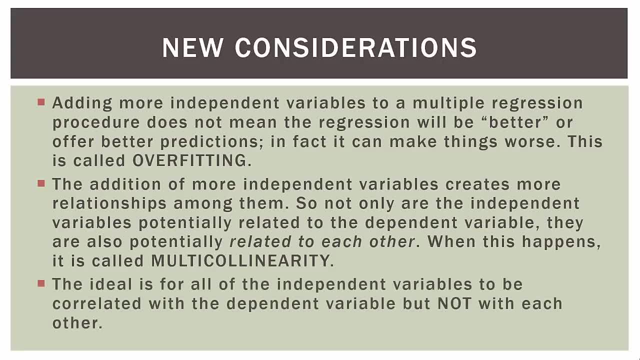 are correlated with each other. So the ideal, the perfect world, is for all of the independent variables to be correlated with the dependent variable, but not with each other. And again, we'll talk about overfitting more as we go We'll talk about multicollinearity. 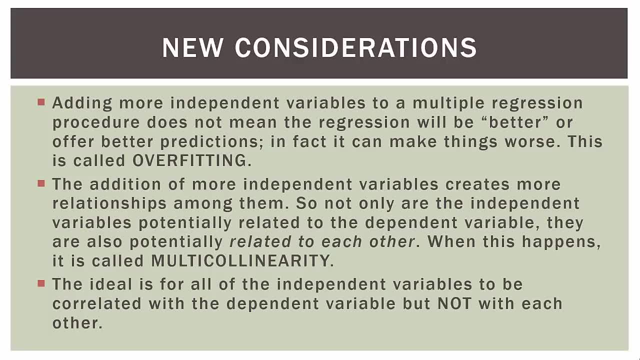 multi-collinearity more as we go forward. And just keep in mind that the ideal is for the independent variables to be correlated with the dependent variable, but not with each other Now because of multi-collinearity and overfitting. 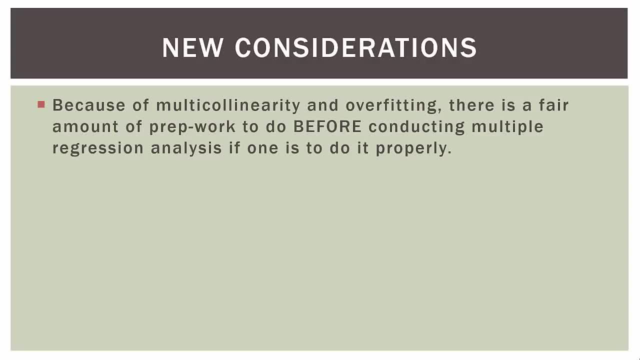 there is a fair amount of prep work to do before conducting multiple regression analysis if one is to do it properly, And in a future video we will walk through all those things step by step so that you form the best model you can. So things like correlations, scatter plots, 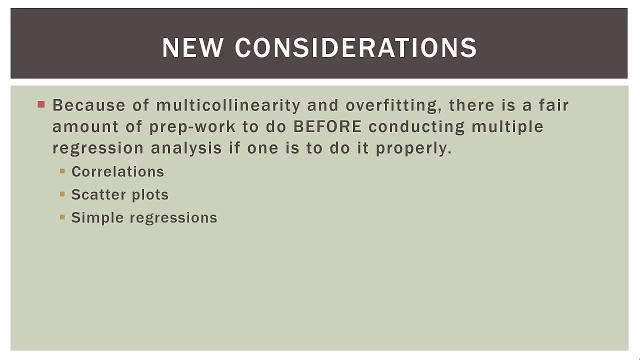 and some simple regressions between the independent variable- each one of them- and the dependent variable, just to see how they're related. So to do multiple regression properly, really running the multiple regression is the very last step. There's a lot of prep work to do before doing that. 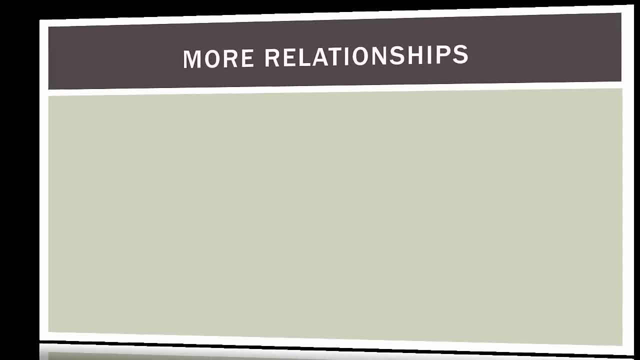 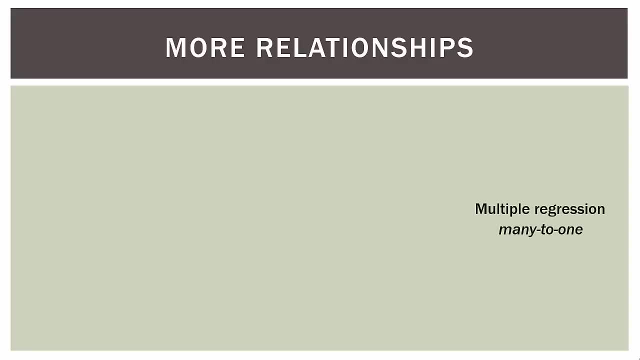 and again. we'll talk about it as we go. So, as we talked about before, adding more independent variables creates more relationships among other variables. So we have this many-to-one relationship. Now in our problem we have a dependent variable, that is, the travel time. 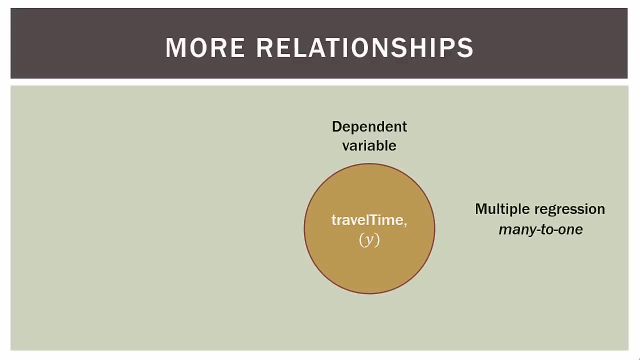 We are trying to predict the travel time of these trips Now. we are utilizing two independent variables that we selected. We have miles traveled, that's our x1, and then we had the number of deliveries, or num deliveries, which is our x2.. 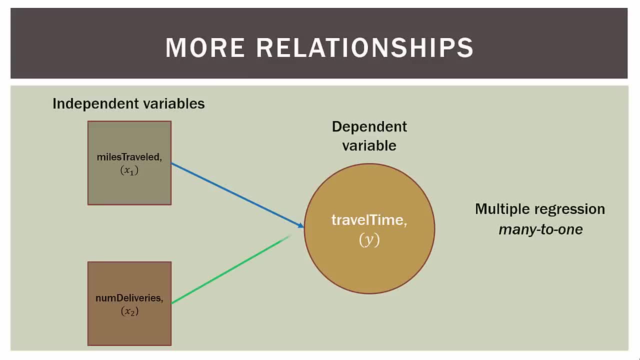 Now we'd like to utilize the number of deliveries and we'd like to utilize those two independent variables to make predictions about the dependent variable. Now, by setting it up this way, we also create a third relationship, and that is the relationship between the two independent variables themselves. 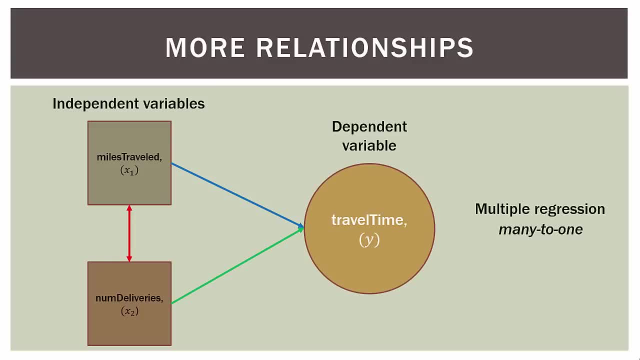 So we don't have just two relationships, independent to dependent. We now have a relationship between the independents and having that relationship sets up the potential multicollinearity risk. So we're going to have to see when we do this problem, whether or not these two independent variables. 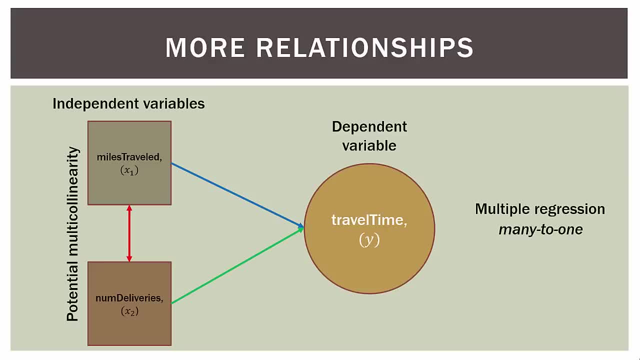 are correlated with each other, And the easy way to think about this is that if these two independent variables are related to each other, we're really not sure which one is explaining the variation in the dependent variable. So if I put sea salt and table salt in my dinner, 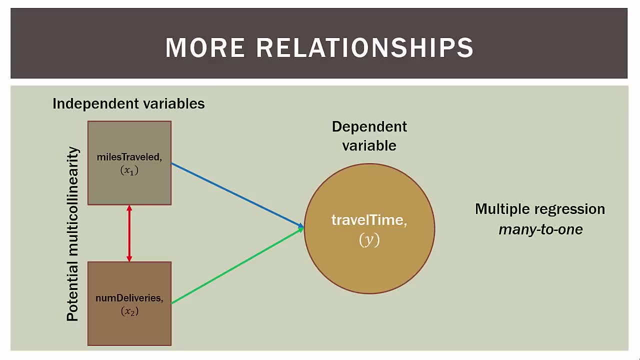 all I know is that it tastes salty, But I can't tell the difference necessarily between the two, because they're both salt. They have the same relationship to my now salty dinner. So we want to have a distinction between the independent variables so they explain something different. 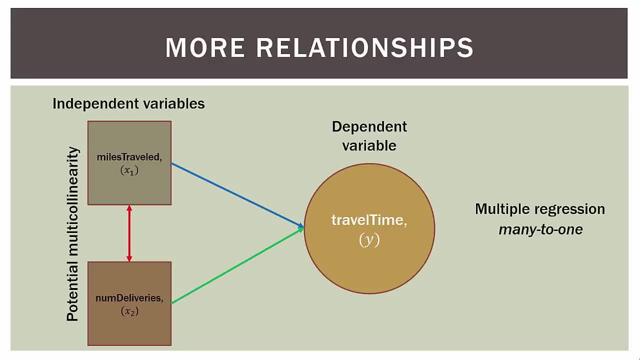 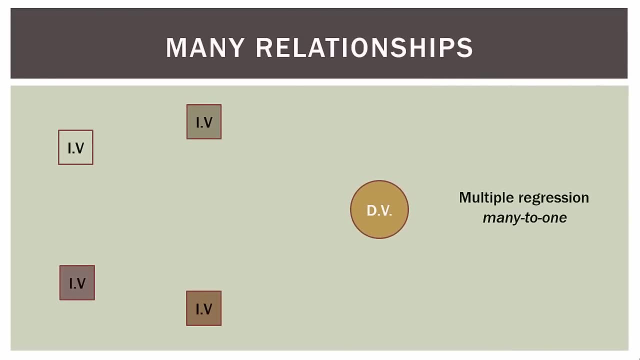 They have a different relationship to the dependent variable over here on the right. So we will walk through that analysis as we go forward. Now let's look at this situation. So here we have one dependent variable and four independent variables. So we know we have the four relationships. 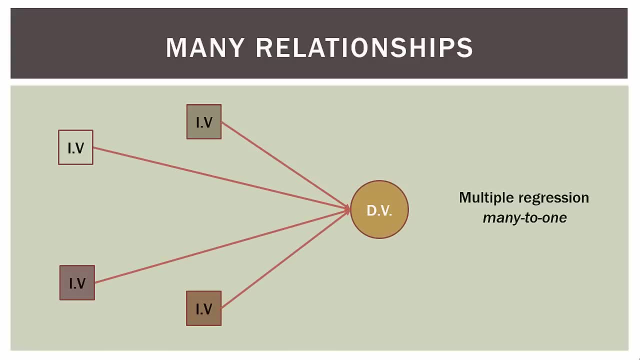 with each independent variable and the dependent variable. So right there, we already have four variable relationships, But we're not done. We have to account for all the relationships between the independent variables, And that's six more. So now with four independent variables and one dependent variable. 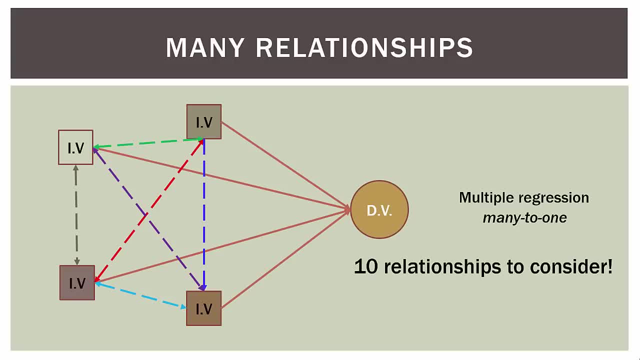 we have 10 relationships we have to consider. Now you can see, as each independent variable is added, these relationships become very numerous. So part of the art of multiple regression is deciding which independent variables make the cut and which do not, And we'll talk about that as we go, of course. 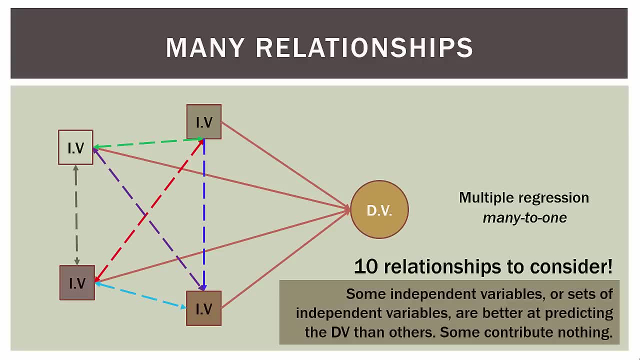 So the bottom line is that some independent variables, or sets of independent variables, are better at predicting the dependent variable than others, And some independent variables contribute nothing. So we'll have to decide which independent variables to include in our model and which ones to exclude. 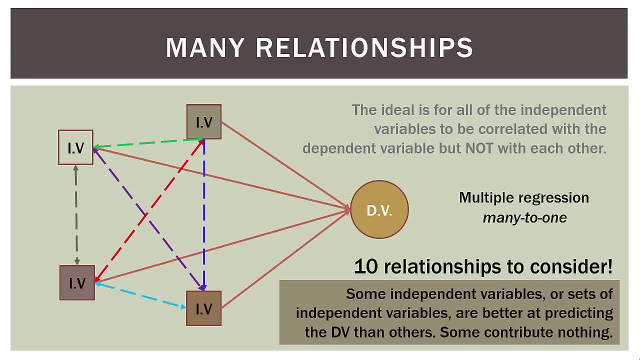 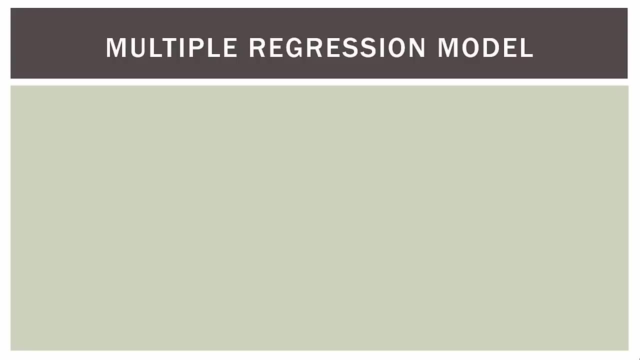 So again, the ideal is for all of the independent variables to be correlated with the dependent variable, so the orange lines, but not with each other, so the colored dotted lines here. So this slide is not something you have to really commit to memory, but I just want to show you sort of 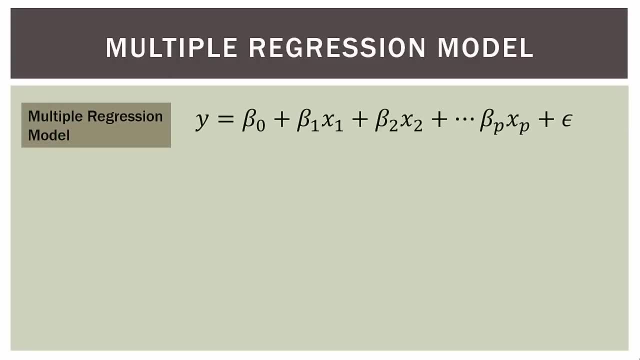 where the multiple regression model comes from. So we have our multiple regression model, which is: y equals beta sub zero plus beta. one x one plus beta, two x two plus, et cetera, et cetera, et cetera. P just means the number of variables we have, plus epsilon. 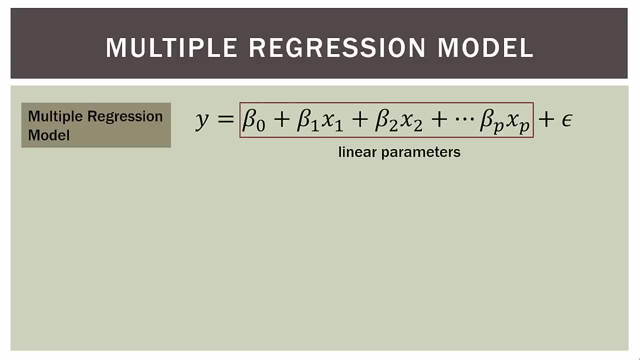 Now, over here on the left, what we have are the sum of linear parameters. So we have beta sub zero, which is our intercept, and then we have beta one x one, which is one variable, and then we have beta two x two. 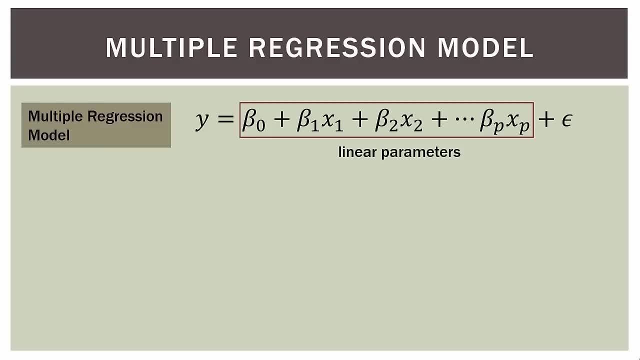 which is our intercept, and then we have beta one, x one, which is one variable, and its weight. then we have x two, beta two, which is another variable, and its weight, et cetera, et cetera. So it's just the sum of some linear parameters. 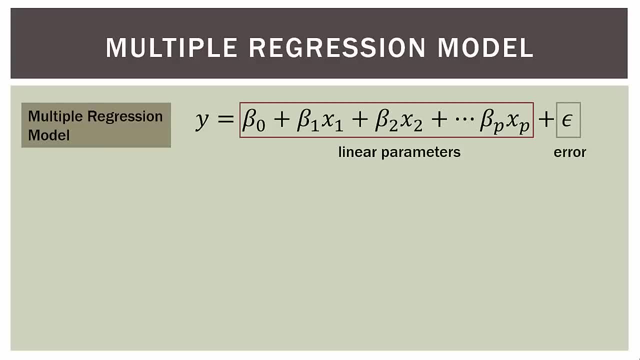 Then over here on the right we have our error term. So we've seen this before in simple linear regression. So we have an intercept plus a set of linear parameters plus an error term. Now for the multiple regression equation. we have the expected value of y. 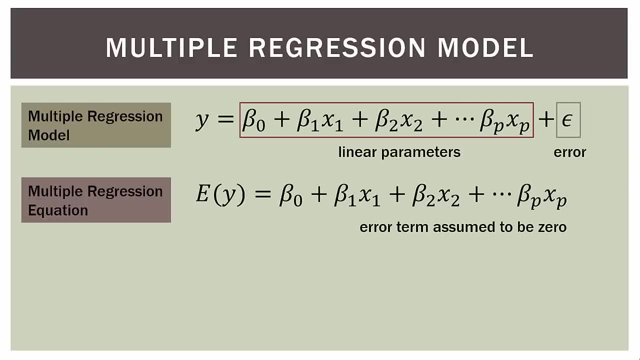 equals everything we see up at the top, but there is no error term. Well, why is that? That's because in the multiple regression equation the error term is assumed to be zero. So zero is zero and therefore it's not on the end. 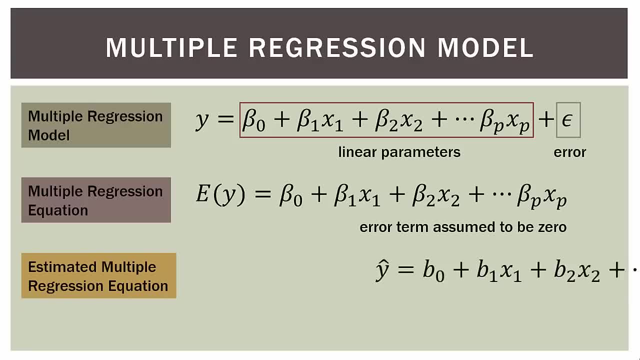 of that equation? Well, the one we're going to be familiar with, and a formula of that equation is the estimated multiple regression equation. So, again, when we're using sample data, it's never going to be perfect. We're estimating, So we have to use the estimator here. 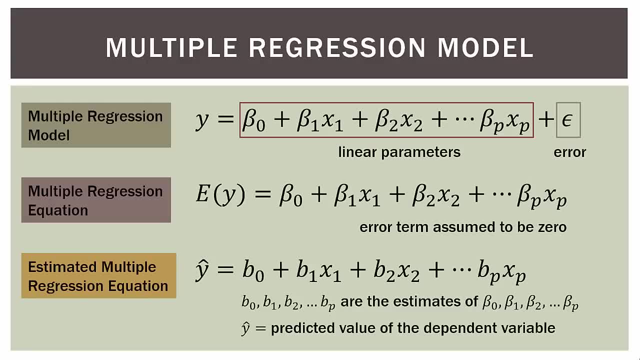 estimated multiple regression equation. So y hat is the predicted value of y equals b sub zero plus b, one x one plus b two x two, et cetera. As you can see, it follows the same form as the multiple regression equation above it. 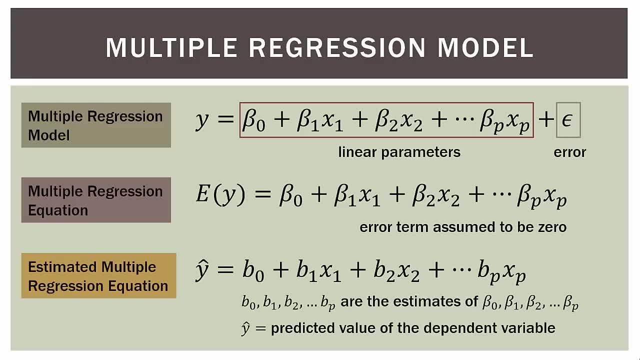 And everything that you see at the bottom is just an estimate of what is above it. So b zero, b one, b two are all the estimates of beta zero, beta one, beta two, et cetera, And then y hat is the predicted value. 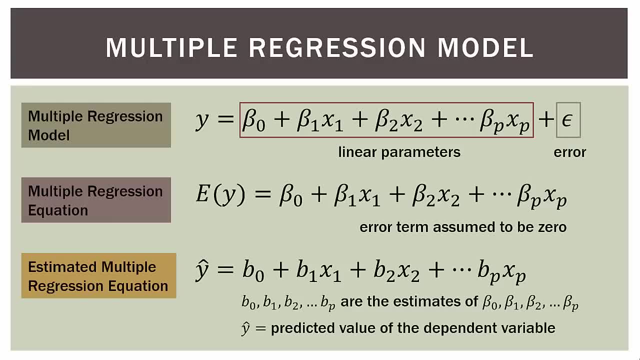 of the dependent variable. So, again, this is not something you need to really commit to memory, but I just want you to see the pattern of how these multiple regression equations are gonna look, and we'll talk about in the next slide sort of what they mean. 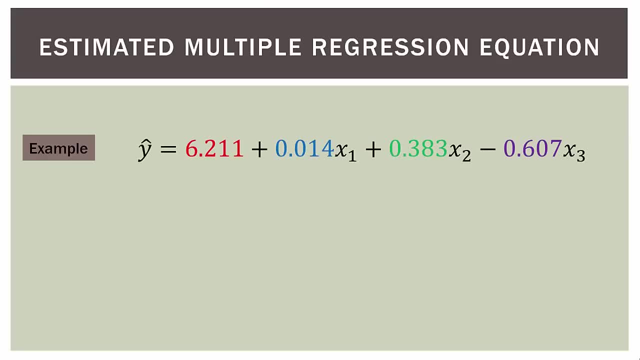 So let's go ahead and look at an example. So this is a multiple regression equation you may generate based on some analysis you conduct. So if y hat equals 6.211 plus 0.014 x one plus 0.383 x two, 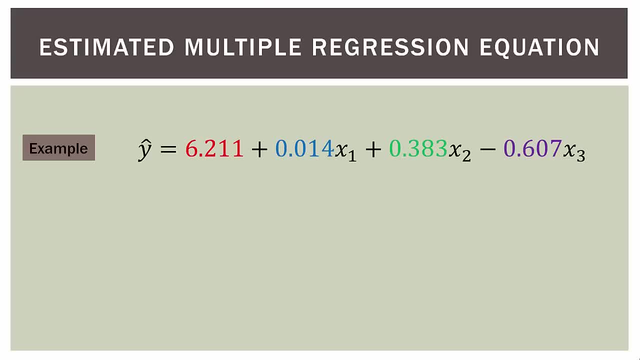 minus 0.65 x zero, seven x three. So this is a standard form of a multiple regression equation you may generate. Now if we look at our estimated multiple regression equation, so we have y hat equals b, zero plus b, one x one plus b, two x two, et cetera. 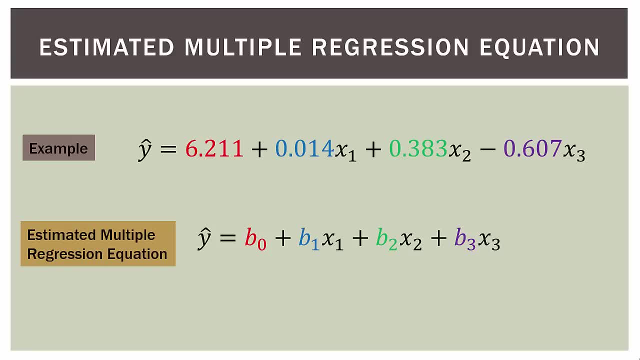 If you look at that and compare it to the equation at the top, you can see that they're very similar. We just have some stand-in numbers that we have to interpret. So we have our variable. so x one, x two and x three. 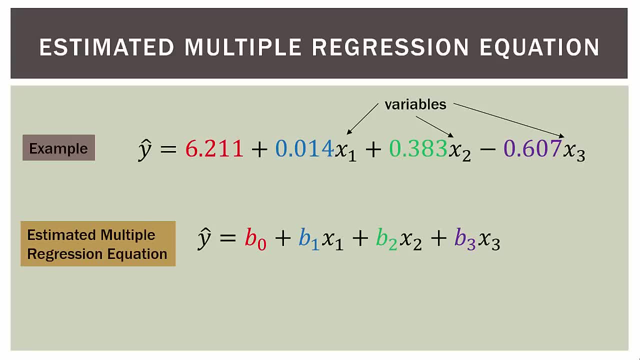 are our variables And we can see that they're in place there at the top and of course in the equation at the bottom. Then we have some coefficients and an intercept. So 6.211 is our intercept, which corresponds with b sub zero in the equation below. 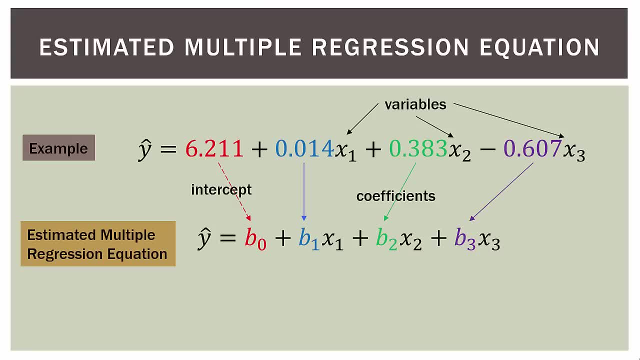 Then we have 0.014, there in the blue, that corresponds to the first coefficient on the bottom, et cetera, et cetera. So we follow the same basic form: Intercept, plus some coefficients paired with 0.014 x one. 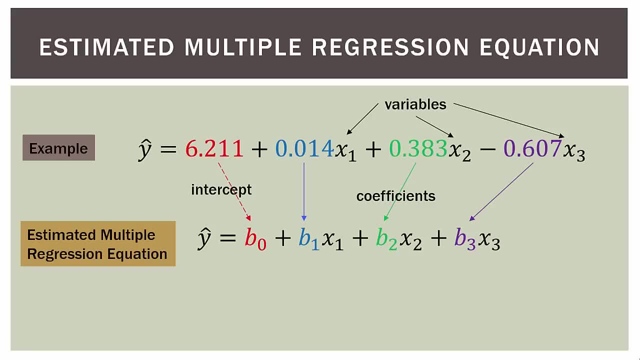 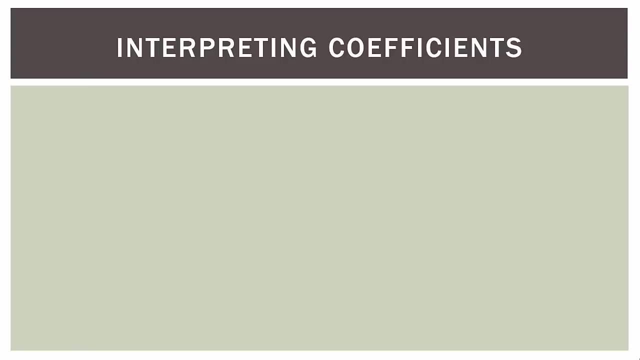 Then we have some coefficients paired with a variable, So coefficient with the first variable, a coefficient with the second variable and, in this case, a coefficient with the third variable. And again, these are all estimates of the multiple regression model. So how do we interpret the coefficients? 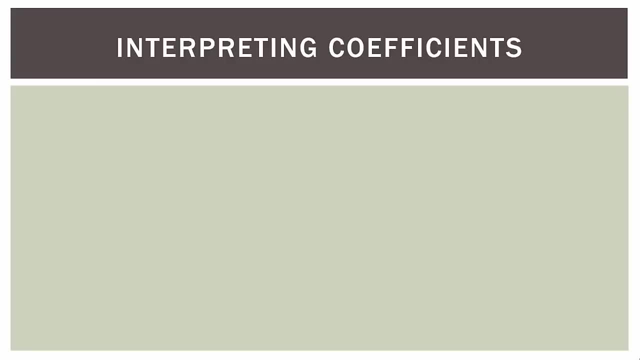 in multiple regression They're interpreted a bit differently than they are in simple linear regression. Let's take this example. So we have y hat equals 27 plus 9x one plus 12x two. Now everything we see here is in thousands of dollars. 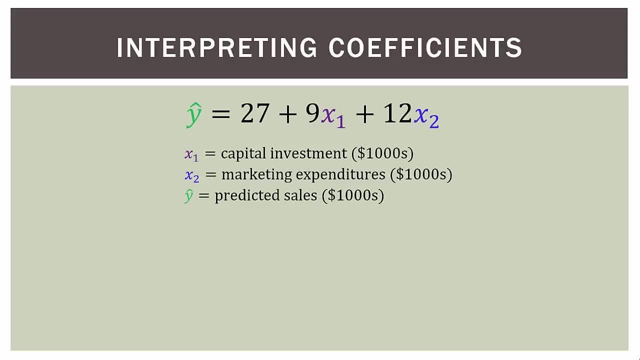 So x one- that's our first variable- stands for capital investment in the thousands of dollars. So x two stands for the marketing expenditures in thousands of dollars that are in the blue And of course y hat is gonna be our predicted sales in thousands of dollars. 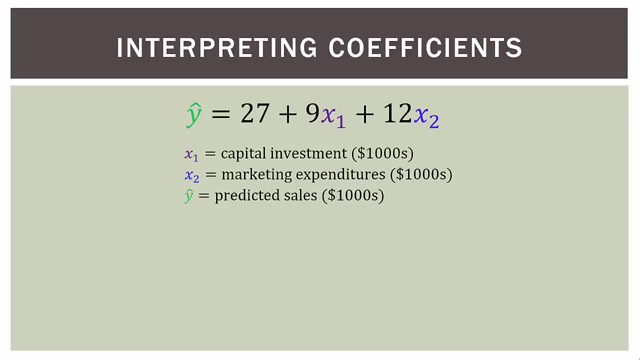 So everything is in thousands of dollars. We have to keep that in mind as we go about interpreting it. So in multiple regression, each coefficient- so we have our nine and our 12 up there- is interpreted as the estimated change in y corresponding to a one unit change in a variable. 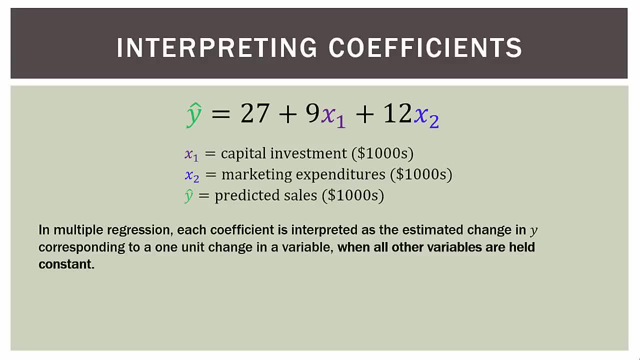 when all other variables are held constant. So what does that mean in this problem? So, in this example, $9,000 is an estimate of the expected increase in sales, which is y, which is Y corresponding to a $1,000 increase. 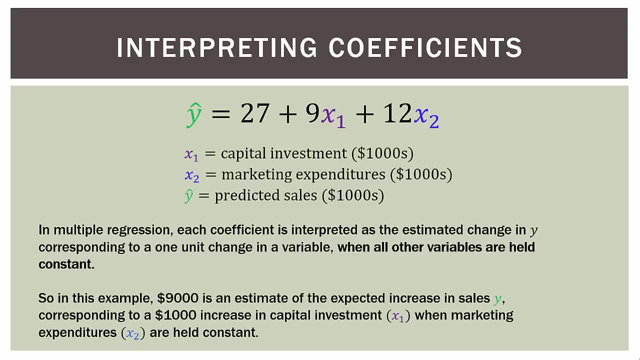 in capital investment, which is our X1 up there. So remember everything's in thousands of dollars, so I'm just making sure it's actually in dollars here at the bottom. So $9,000 is an estimate of the expected increase in sales. 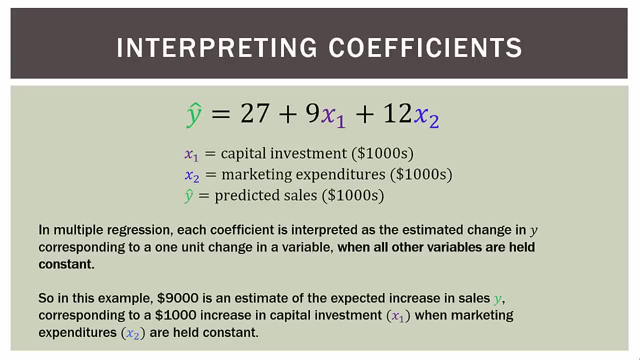 corresponding to a 1,000 increase in capital investment, which is X1.. Well, why is that? Look at the coefficient with our X1 variable. up there It is nine. So if we increase X1, where X1 is the number one, 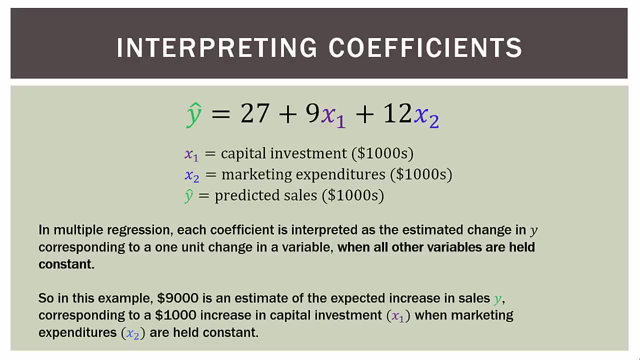 we have nine times one, so that's nine times $1,000.. That's $9,000.. Assuming we hold the X2 over here on the right constant and that's how we interpret the coefficients in multiple regression, We could flip that and say: 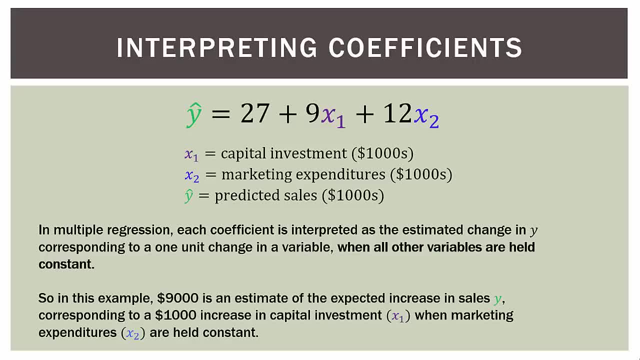 well, $12,000 is $9,000.. $9,000 is an estimate of the expected increase in sales Y corresponding to a $1,000 increase in marketing expenditures when capital investment is held constant. So a one unit increase when everything else. 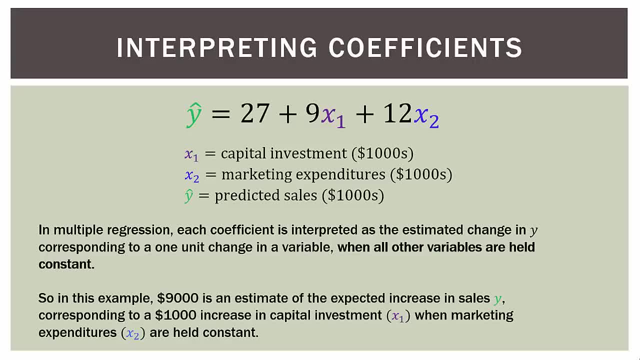 all the other variables are held constant And, again, we'll be doing this more in future videos, so we'll get some practice at it. but that's the basic idea of how we interpret coefficients in our multiple regression equation, So let's go ahead and do a quick review. 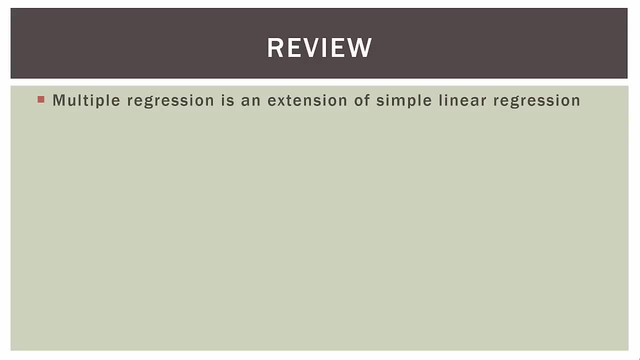 and then we'll be done with this first video. So multiple regression is an extension of simple linear regression. Two or more independent variables are used to predict or explain the variance in one dependent variable. Two problems may arise, however: overfitting and multicollinearity. 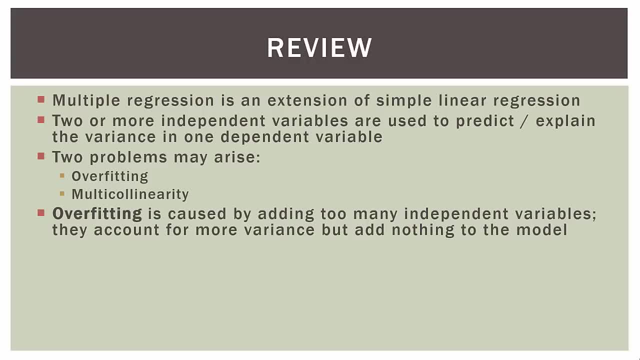 So overfitting is caused by adding too many independent variables. They account for more variance, but you know, but really add nothing more to the model. Then multicollinearity happens when some or all of the independent variables are correlated with each other. 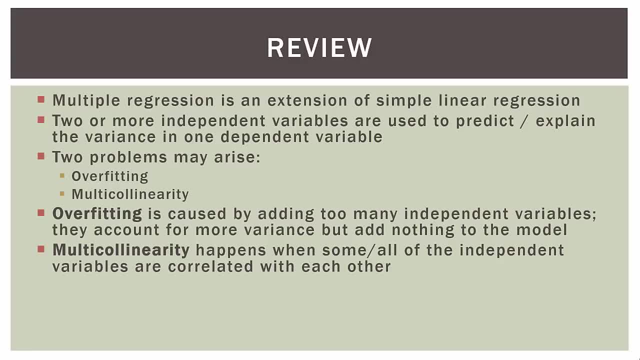 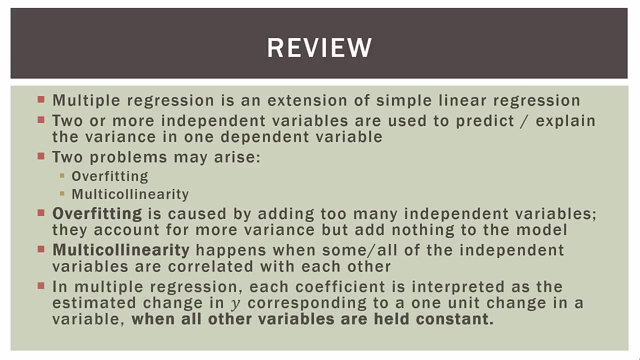 and it becomes hard to tell which is actually predicting or explaining the variance in the dependent variable, because they're so similar. In the multiple regression, each coefficient is interpreted as the estimated change in y, the dependent variable, corresponding to a one-unit change in a variable. 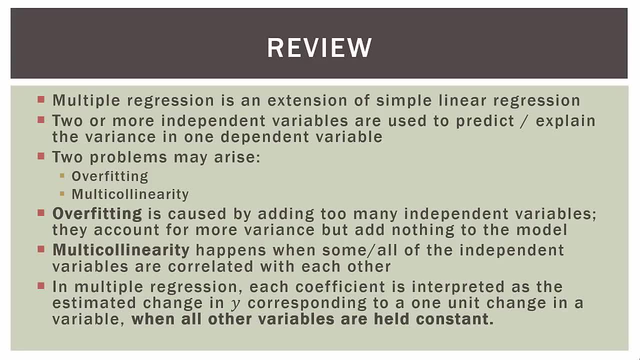 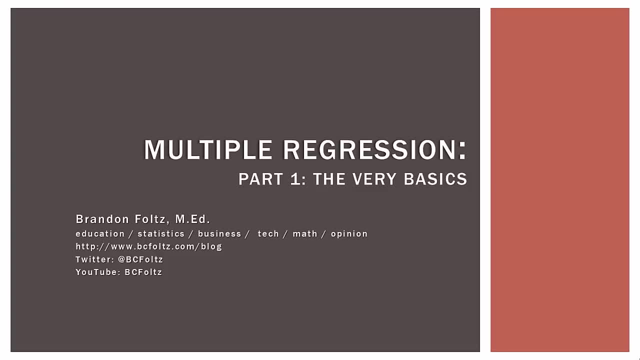 when all other variables are held constant. And again, we'll practice that more as we go. So this was our first video, just the very basics of multiple regression. We'll be doing more videos in the future and walking through the process by which we examine our variables. 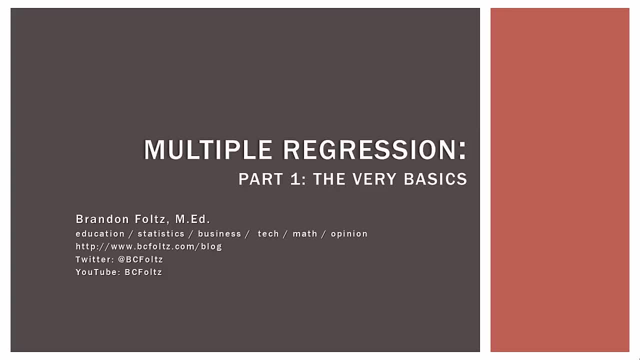 We look at relationships among them before we even ever get into conducting the multiple regression using a statistics pattern. So we'll be doing a lot of pre-work to see what we can do in the next video. So I hope you found this first video helpful.